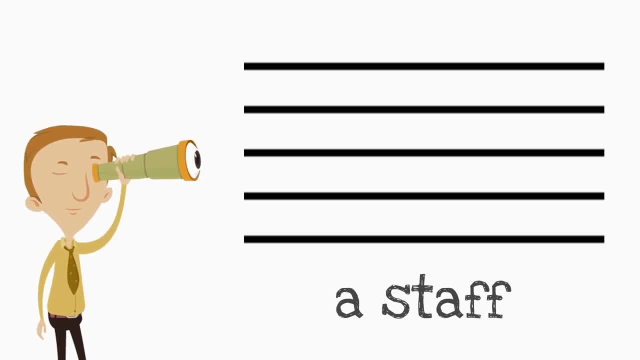 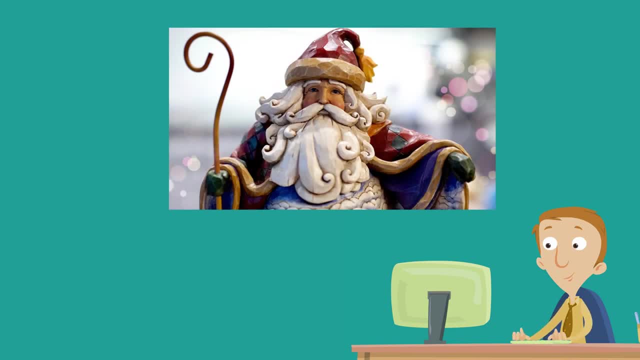 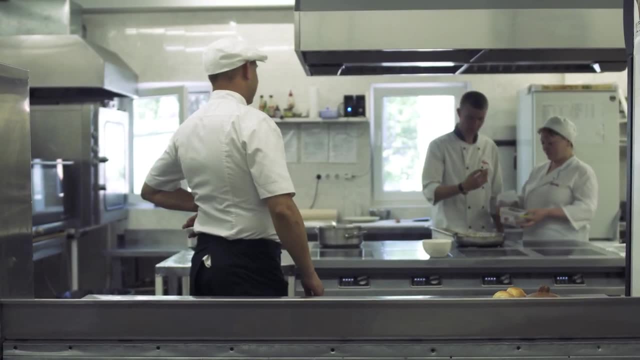 thinking: I know what a staff is. That doesn't look like a staff to me. Maybe when you hear the word staff, you think of a walking stick, For example- this is a staff. Or maybe when you hear the word staff, you think of people who work together in a company or an organization. Well, 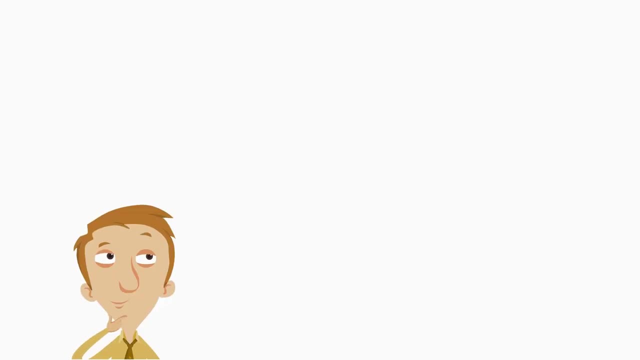 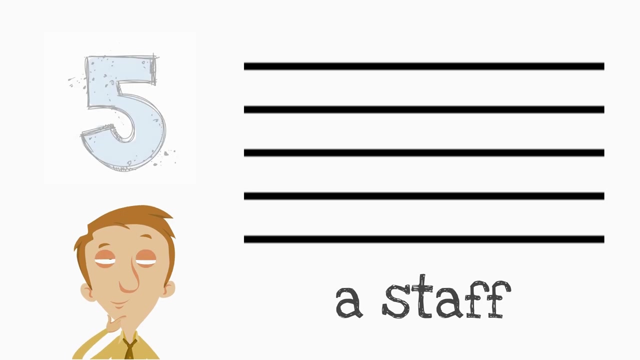 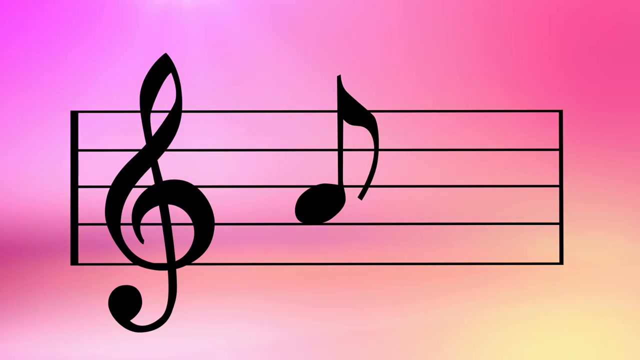 that is called a staff too. Staff can mean many things. In music, these five lines are called a staff, And a staff is always five lines, Never four or six, Always five. Ooh, here we have another staff. We know it's a staff because it's got five lines. But what are these symbols? What do these? 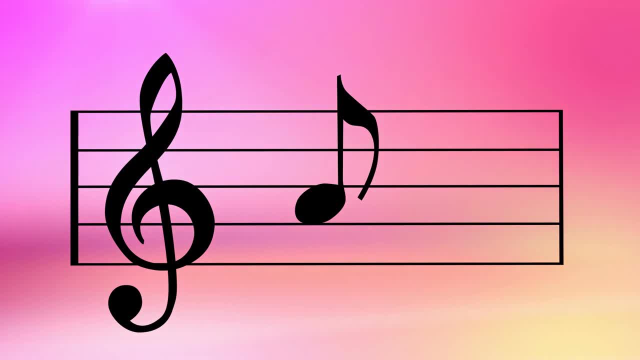 symbols mean. Well, this first symbol is called a treble clef. Wow, that's interesting, A treble clef, Can you say treble clef, Treble clef, Wow. This other symbol is a note, A musical note. Okay, so this symbol is called a what? Yeah, a treble clef And notice. 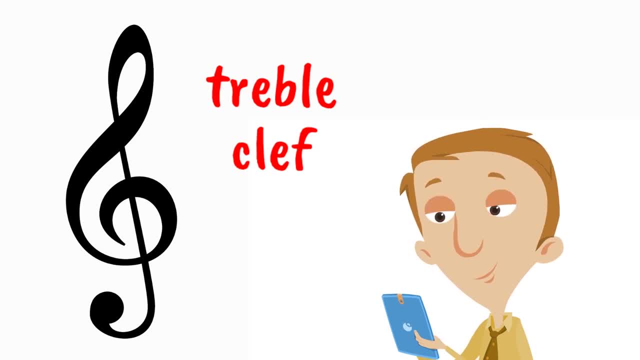 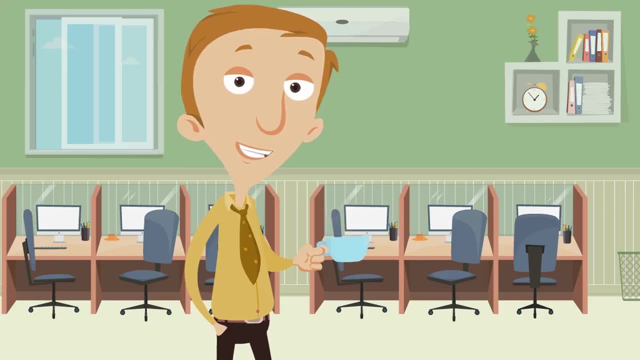 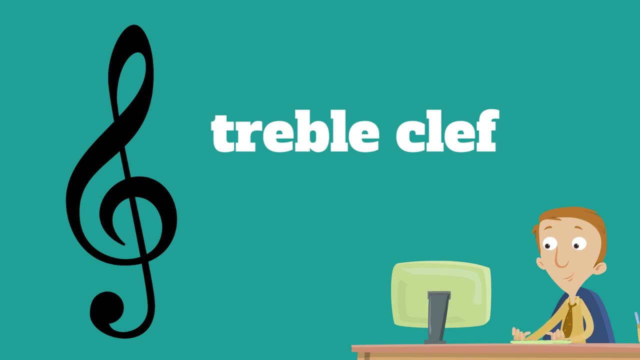 a treble clef almost looks like a G, doesn't it? That's an interesting symbol. This musical symbol is called a treble clef. Okay so, this musical symbol that looks like a G is called a treble clef. Cool, But what does it actually do? 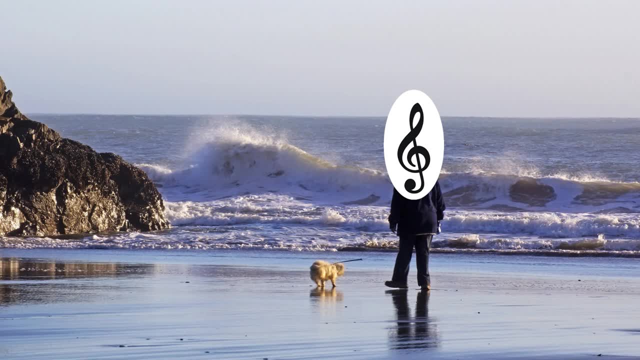 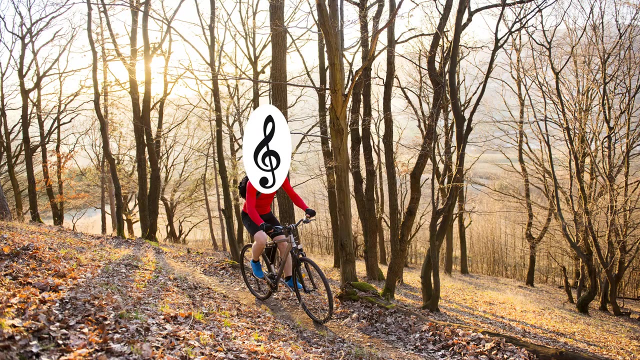 I mean, does a treble clef take its dog on relaxing walks on the beach, enjoying the waves, the sun and the exercise? Or does a treble clef go on long bike rides, exploring trails and racing past plants and woodland creatures along the way? Or does a treble clef read for hours? 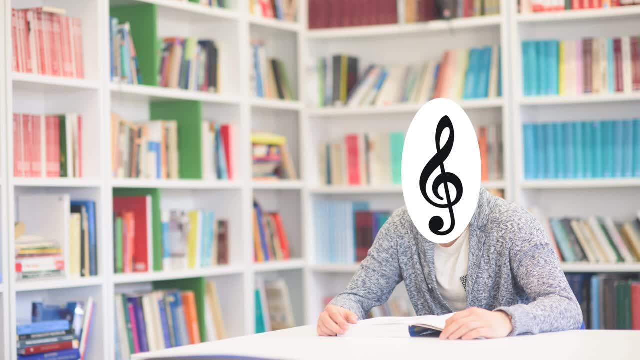 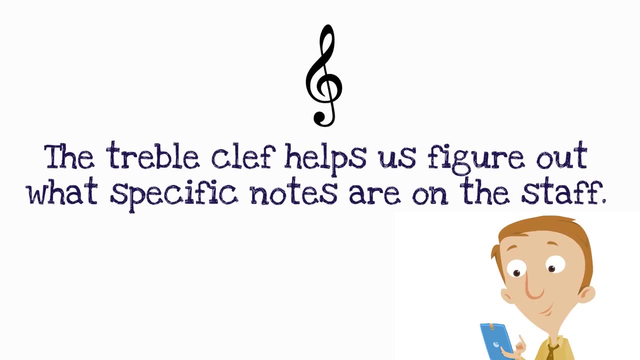 Because the treble clef knows that with the tools we get from learning, we can make a huge difference In this world. No, but that would be awesome. Actually, the treble clef helps us figure out what specific notes are on the staff. That is what the treble clef's job is, and it's an important one. It helps. 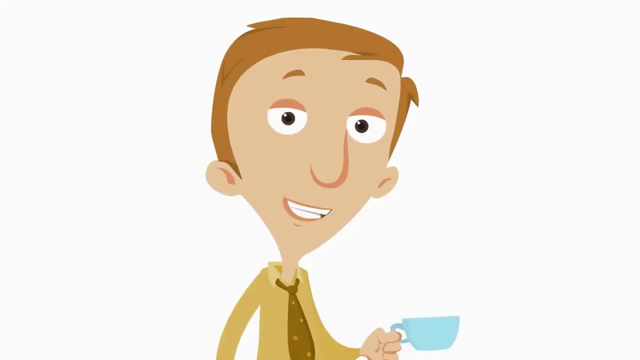 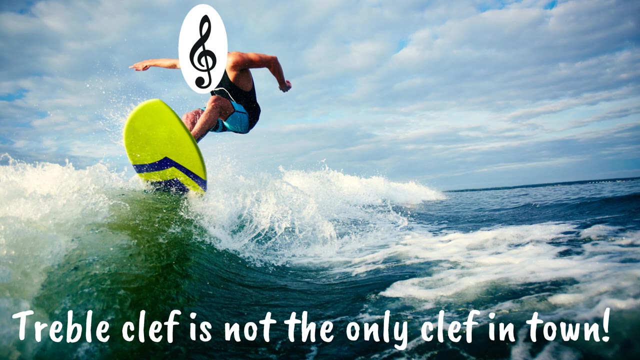 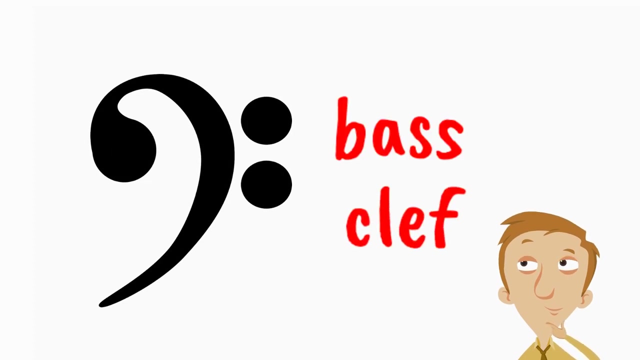 us figure out the notes. The reason it is so important is because treble clef is not the only clef in town. Uh-oh, This musical symbol is called the bass clef. This is what the bass clef looks like. The bass clef. 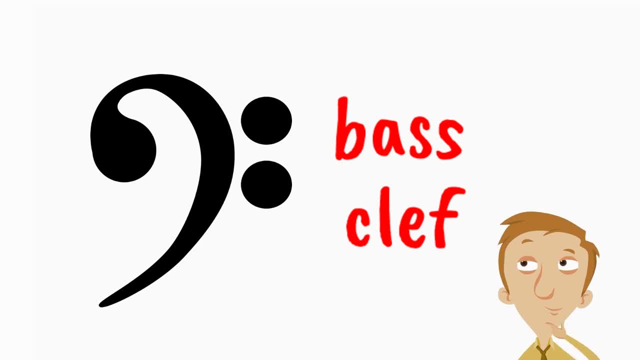 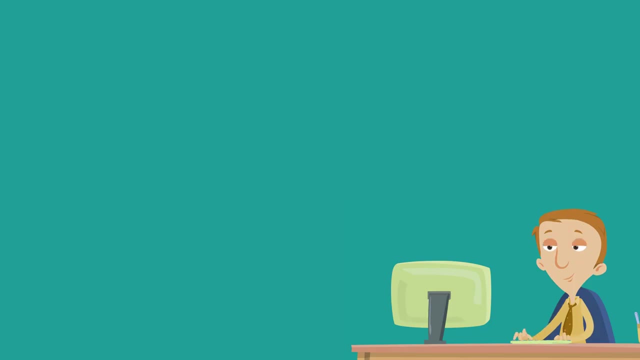 almost looks like an ear with two dots on the outside. The notes on the bass clef are much lower and the notes are different line by line than the notes on the treble clef. Okay, let's review some of what we've already learned. 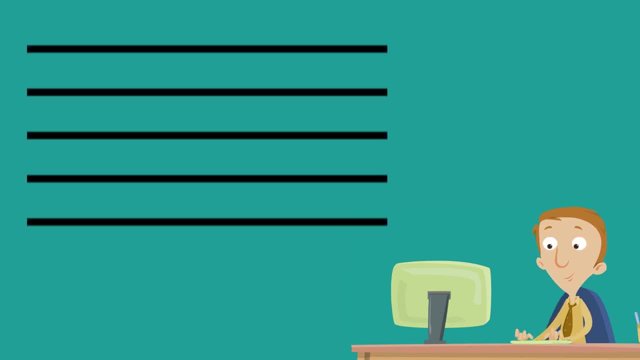 What is this called? Yes, a staff, A staff. Now, look really closely at the staff. Take a picture of it with your mind. We are going to ask you a question about it in just a moment. Okay, How many lines are on a staff? How many lines are on a staff? 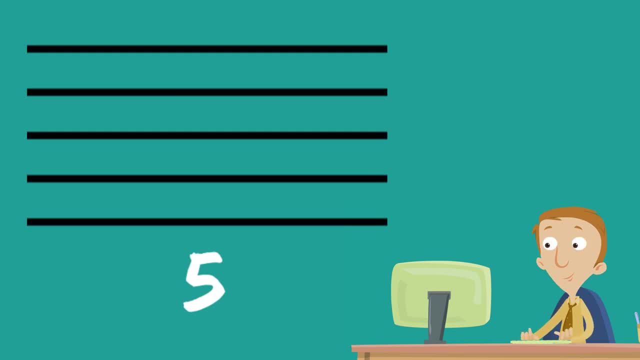 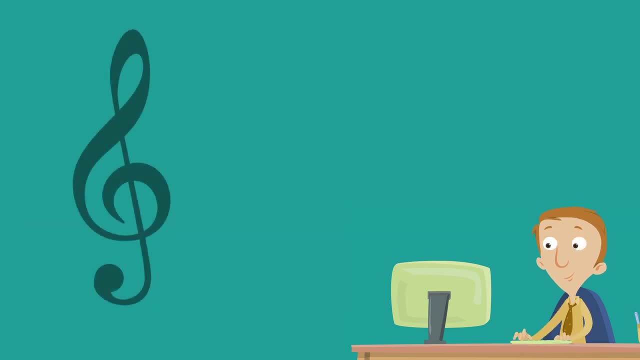 Uh-huh, There are five lines on a staff. A staff has five lines. That's great, All right. What is this musical symbol called? Yes, it is the treble clef. The treble clef. Remember the treble clef. 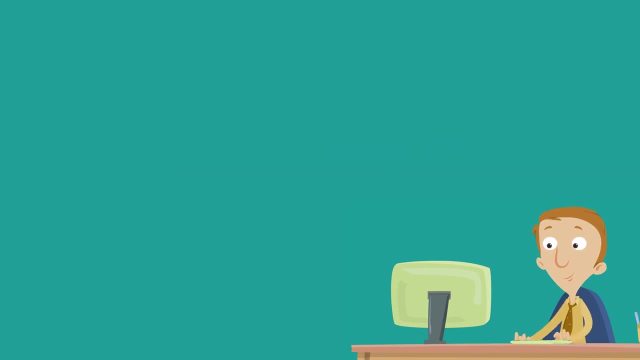 kind of looks like a G- Great. How about this symbol? What is this called Wonderful? The bass clef, The bass clef. The bass clef looks like an ear with two dots on the outside. You did an awesome job. Way to go. 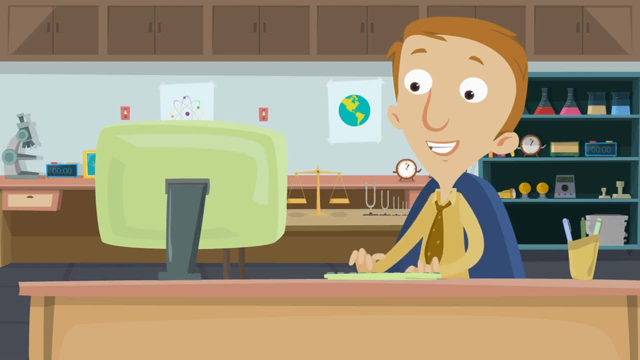 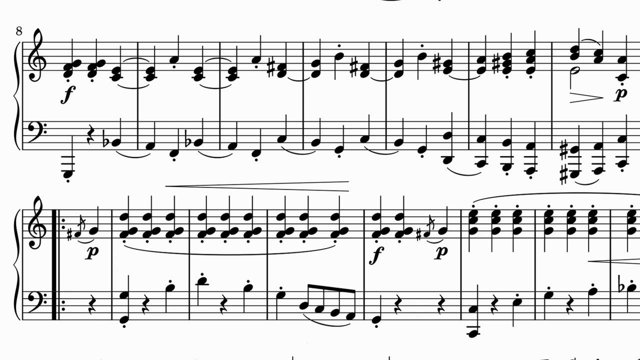 Okay, now we are going to put what we've learned together and look at some actual music so we can learn even more. First, notice all of the staffs. There are four staffs here. They are in groups of two. Each group has the treble clef on the top staff and the bass clef on the bottom staff. 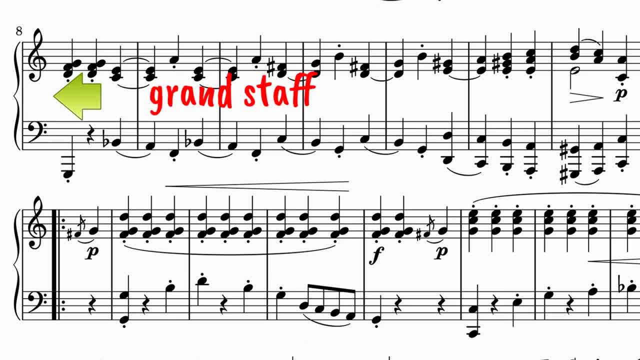 When two staffs are connected, they are called a grand staff. A grand staff. There are two grand staffs on the screen. That's pretty cool. Now you might have noticed some letters on the screen. That's a little strange, right. 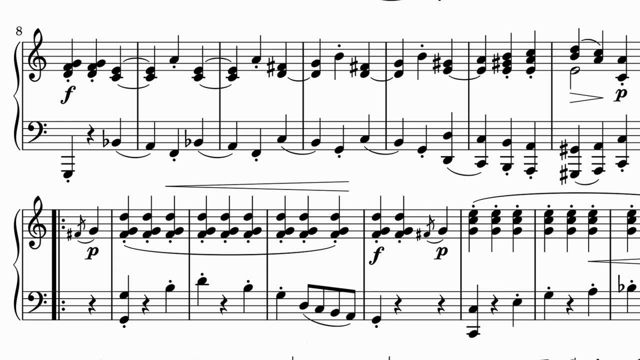 What letters do you see in this music? Yes, the letters F and P. These letters are really special in music. They tell you how loud or how soft the music should be played. The letter F is short for forte. Forte means loud, Loud. 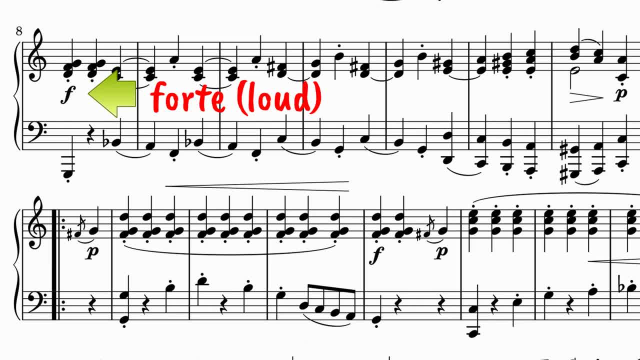 So when you see the letter F in music, it is telling you to play the music LOUDLY. The letter P is short for piano. Piano is not only an instrument, It can also mean playing softly. So when you see the letter P in music, the music is telling you to play softly. 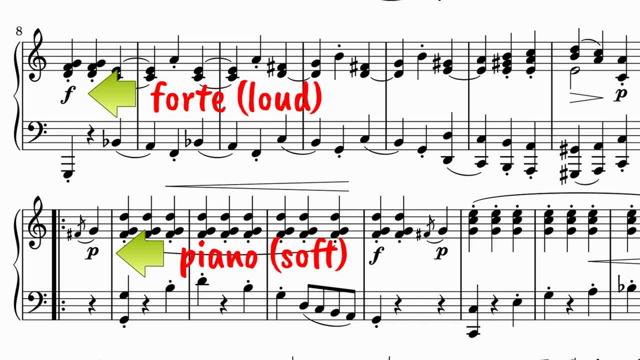 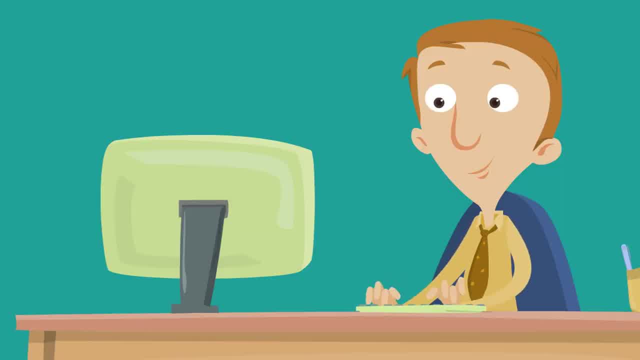 P is short for piano. Piano means playing softly. The letter M is also sometimes used along with just the sound of shells, And it is important for piano. All this involves writing styles as well as voicing heresies, So that's what's so special about this music for piano. It is important to keep in mind that when you're worried about feeding streets or tongues, 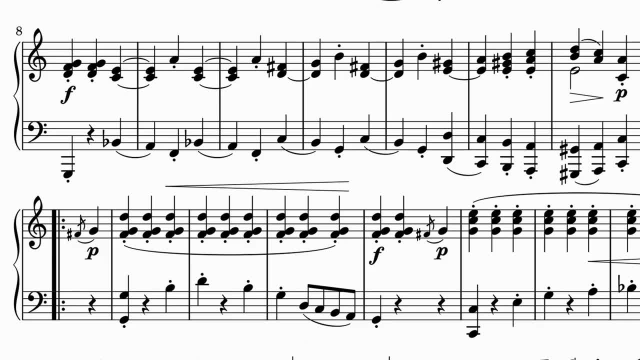 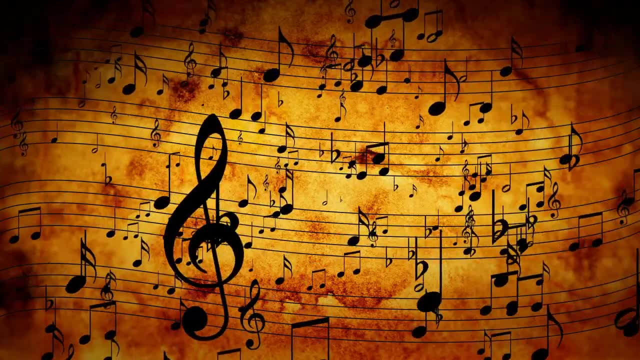 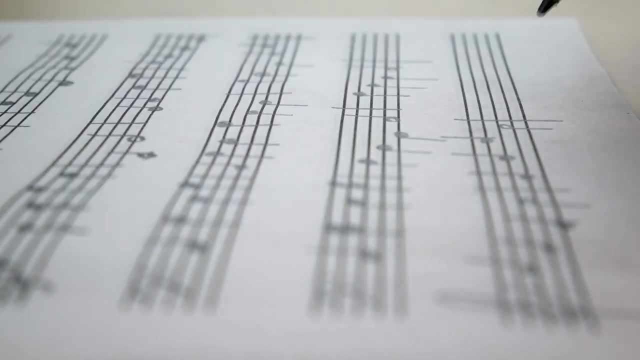 along with the P and the F, or you may see more than one piano or more than one forte. it can vary, but remember F means play loudly and P means play softly. okay, now it's time to talk about notes, notes. you need notes to play music. notes live. 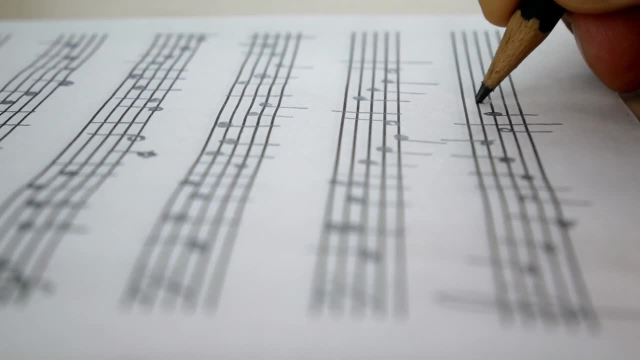 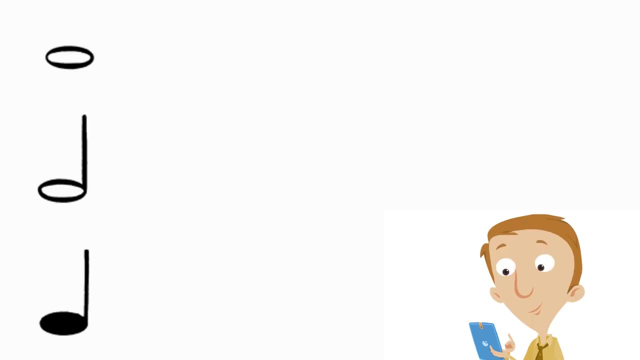 on the staff. there are lots of different types of notes, but in this video we are just going to learn three. the type of note tells you how long the note is to be played. the top note is called a whole note, which makes sense. it has a big hole. 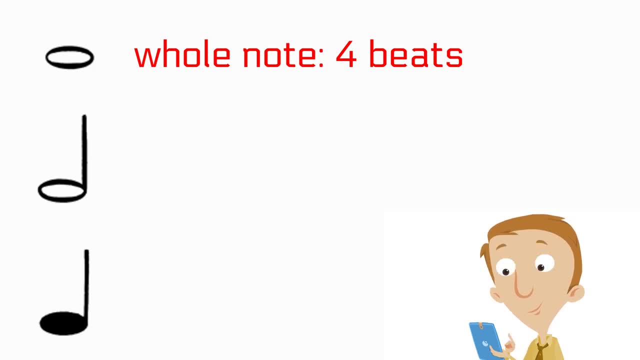 in it. a whole note lasts four beats or claps. the middle note is a half note. it looks like a whole note but it's not a whole note, except it is attached to a long stem. a half note lasts two beats. it is played half as long as a whole note. the bottom note is a quarter note. it looks like a. 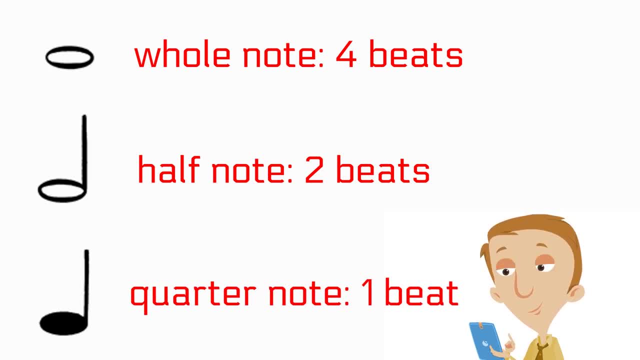 half note, except the hole is filled in. it lasts just one beat. let's listen to each one and you will be able to hear the difference. here is a whole note. okay, here is a half note and a quarter note. it looks like a half note, but it's not a whole note. 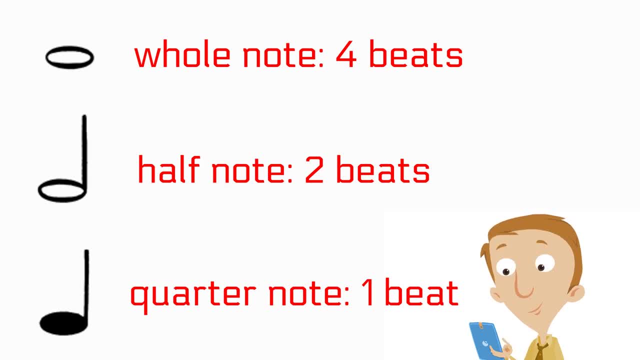 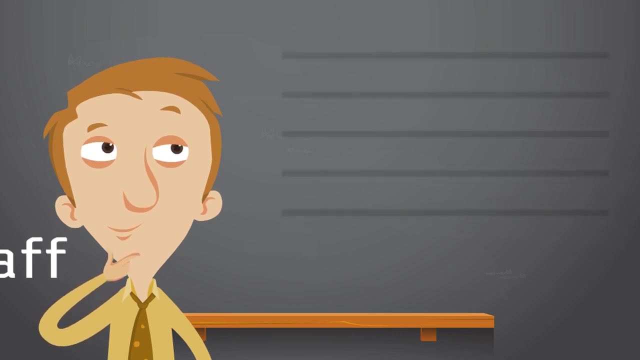 Here is a half note- great. And here is a quarter note- yeah, One more time: a whole note, a half note and a quarter note- awesome. Okay, we've learned so much in this video. We learned that this is a staff. 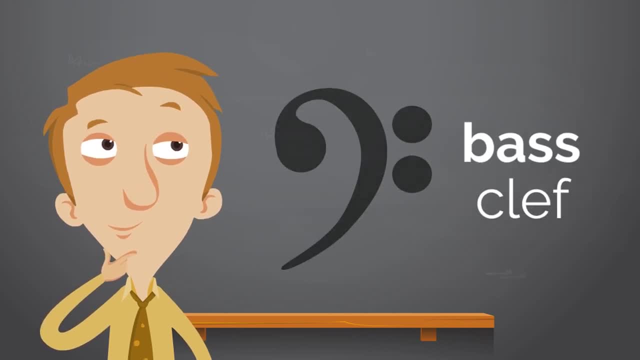 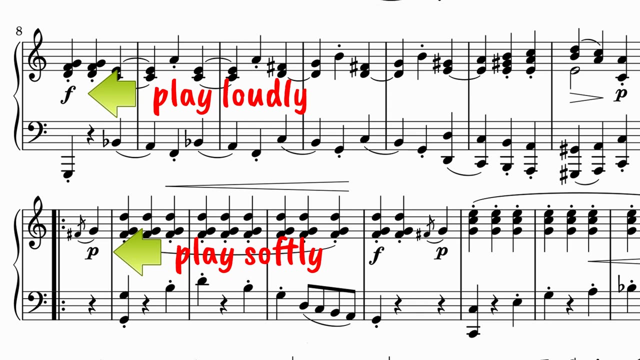 This is the treble clef And this is the bass clef. We learned that in music, P means play softly and F means play loudly. We learned that when two staffs are connected it is called a grand staff, And we learned three types of notes. 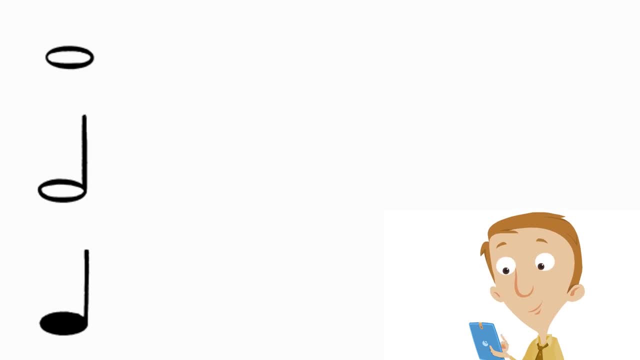 This top note is what type of note? Yeah, a whole note. It lasts four beats. What is this middle note? Uh-huh, a half note. A half note is two beats long. And what is this bottom note? Great, a quarter note. 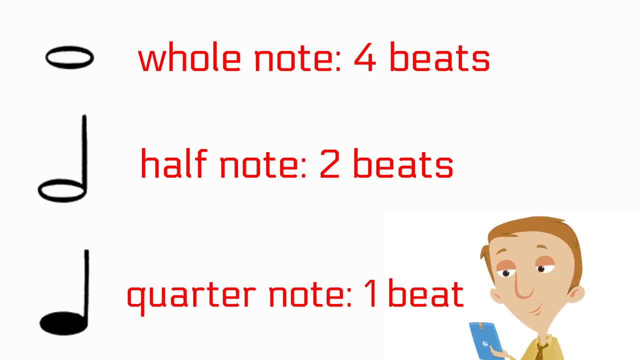 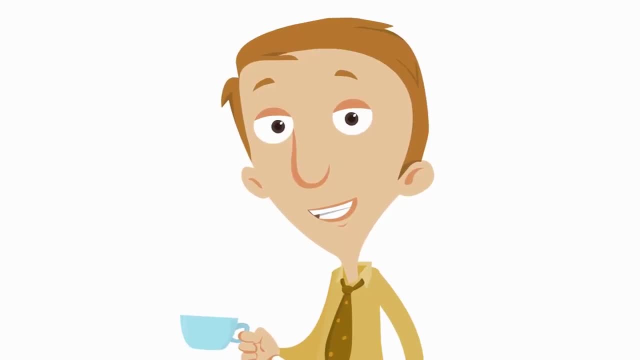 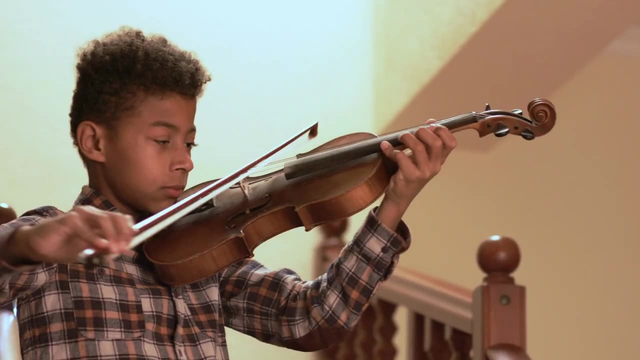 Yes, a quarter note is only one beat. There is so much you can learn about music In this video. we just talked about some music basics. We hope you had fun And that this will be the beginning of a great adventure learning about music. 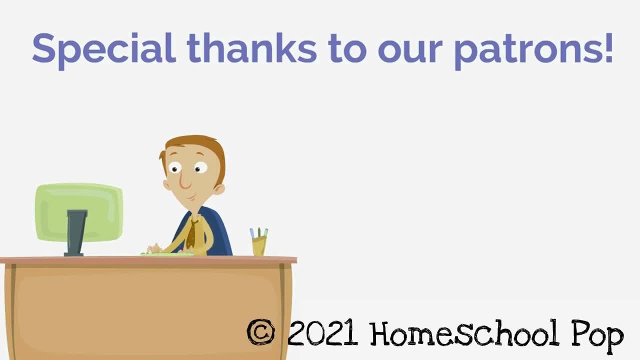 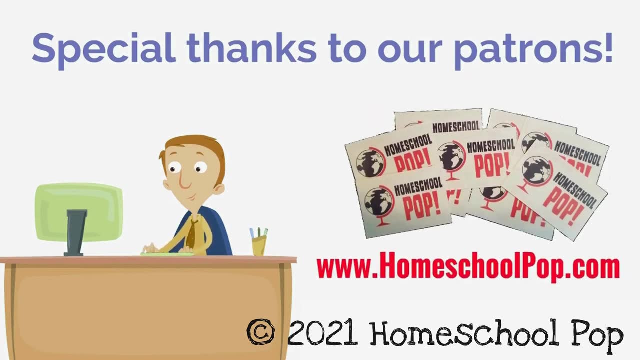 As always, special thanks to our patrons. We appreciate your support so much. If you would like to be one of our patrons and get some Homeschool Pop tattoos, just click the link below this video or visit homeschoolpopcom. We hope you had a great time learning with us. 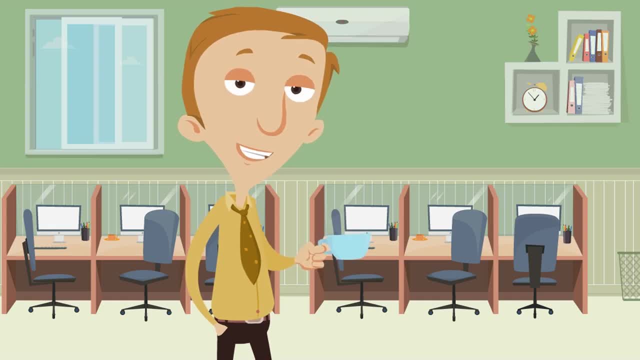 You are so awesome. We'll catch you next video. Bye.